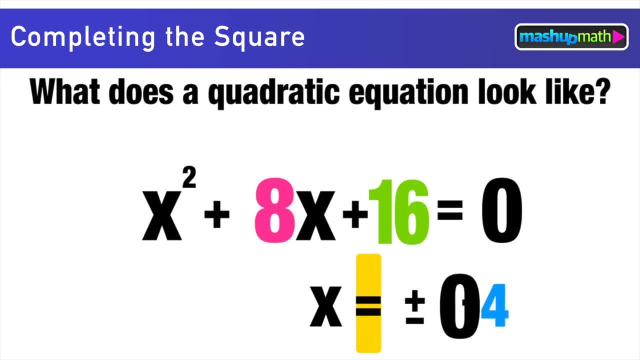 I'm going to rearrange that plus or minus zero minus 4.. And now I can just evaluate: obviously, negative 4 plus zero just equals negative 4.. And negative 4 minus zero also equals negative 4.. So we have one solution. 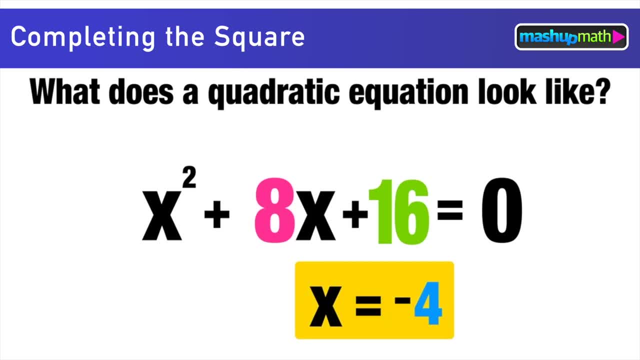 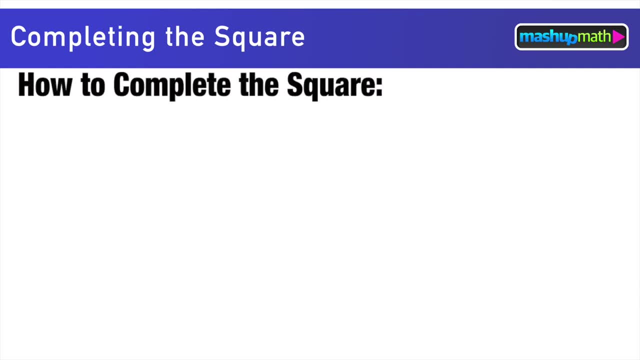 To this quadratic x equals negative 4.. Now, keeping this approach in mind, let's go ahead and learn how to complete the square. So let's go ahead and jump into an example where we have to complete the square in order to solve a quadratic equation. So, for this example, we have x squared minus 6x plus 9. 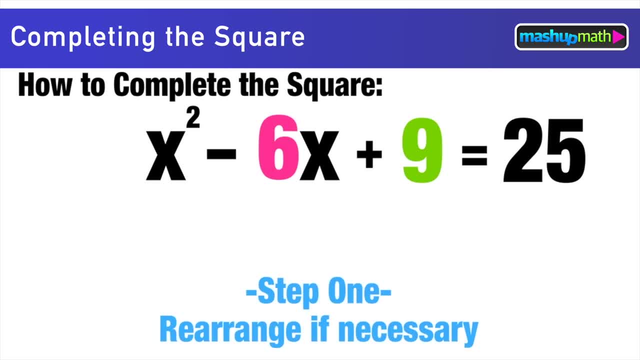 equals 25.. Now our first step here is to rearrange the quadratic, if necessary, And this one. we have to rearrange The constant term, So we have the plus 9.. We want to move to the right side of the equal sign. We want 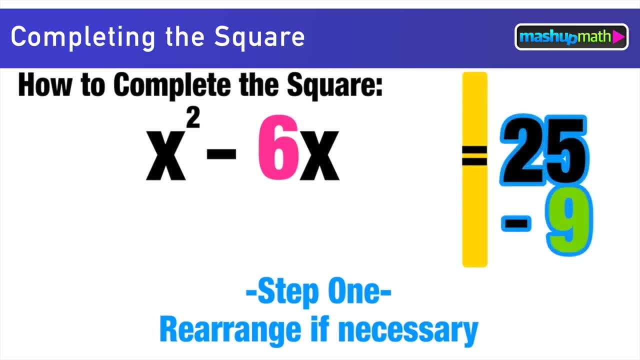 all the constants on one side. So I subtract 9 from the left side, Cancel it out. Subtract 9 from the right side. 25 minus 9 equals 16.. And now my quadratic is arranged the way I want it to be: x squared minus 6x equals 16.. 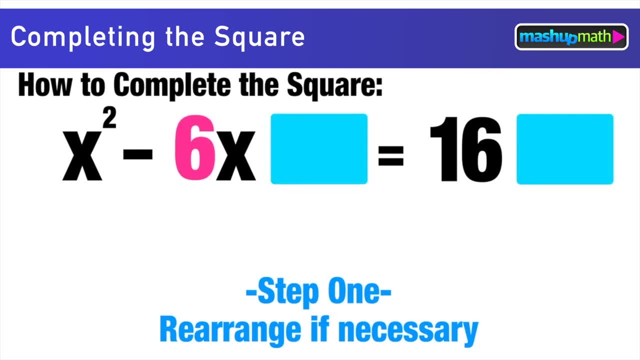 Also note that I'm going to leave these open spaces in the equation. I'm going to use them later on when solving this. Okay, so step two now for completing the square is to add b over 2 squared to the square plus 9.. 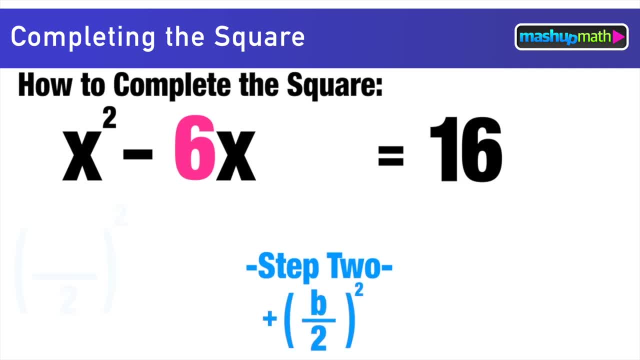 Now what that means is we take the b term, we divide it by 2 and then square that value and add it to both sides. In this case, b is negative 6.. Negative 6 divided by 2 is just negative 3.. And then negative 3 squared equals positive 9.. So we're going to add 9 to both. 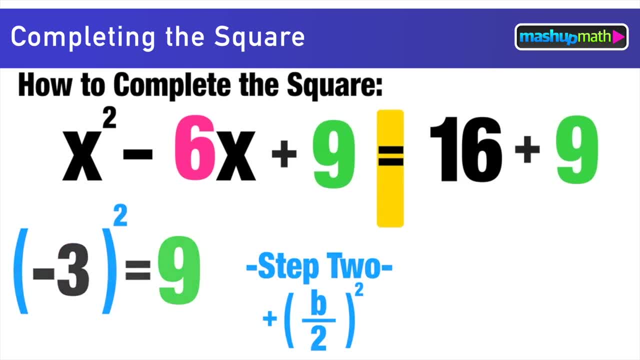 sides of this equation. And now our third and final step for completing the square is to factor and solve for x. So we'll start with the trinomial on the left side of the equal sign: x squared minus 6x plus 9.. Which factors out to x minus 3 times itself, x minus 3.. Now the whole point of completing. 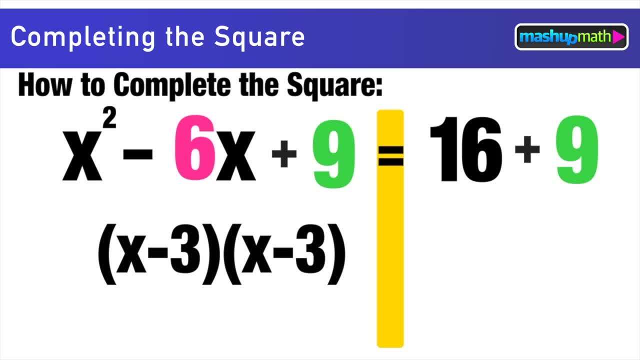 the square is, just like in the last example, to factor out a trinomial in this way, where the factors are the same number, because then we can solve the quadratic using square roots. Now, over on the right side of the equal sign, 16 plus 9 just equals 25.. And back on the 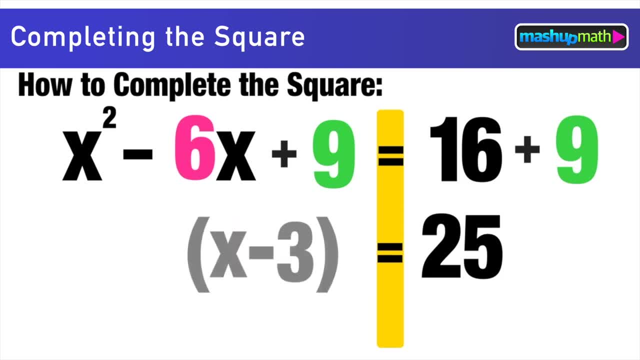 left side. rewrite x-3 times x-3 as x-3 squared. Now to get rid of that 2 in the exponent, I take the square root of both sides. On the left side they cancel each other out. On the right, 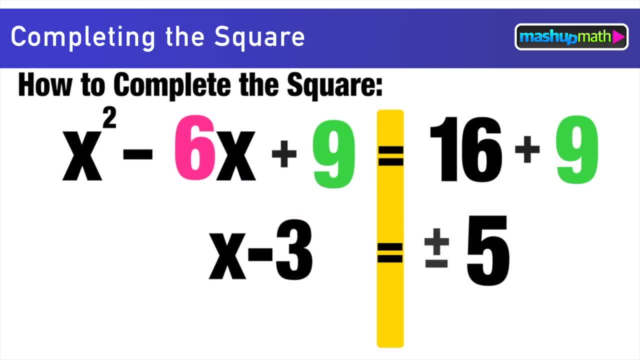 side, the square root of 25 will evaluate to plus or minus 5.. Now our goal here is still to get x all by itself, so we have to get rid of that minus 3 on the left side. I'm just going to add 3 to both sides. Left side: the 3s get cancelled out and now x is all. 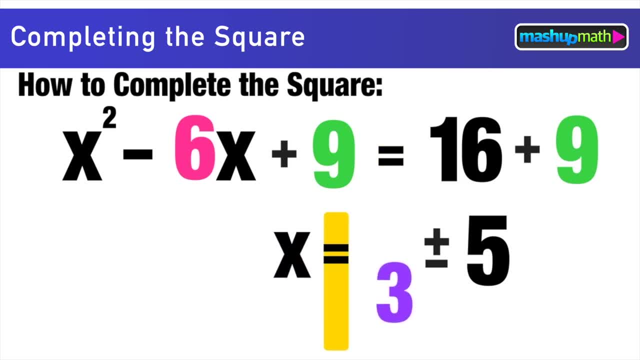 alone. Now we have to go ahead and evaluate the right side and we'll be finished. So first we'll start with 3 plus 5,, which just evaluates to positive 8. That's our first solution for x And our second solution: 3 minus 5, equals negative 2, and we have our 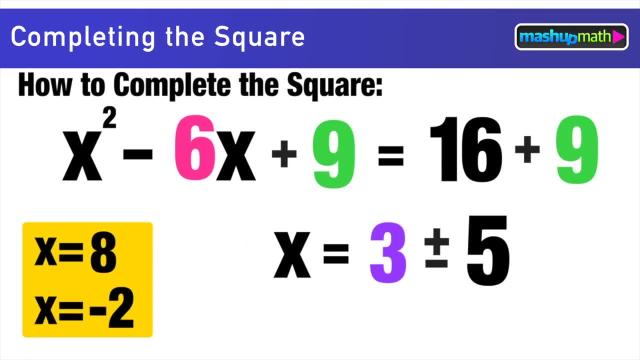 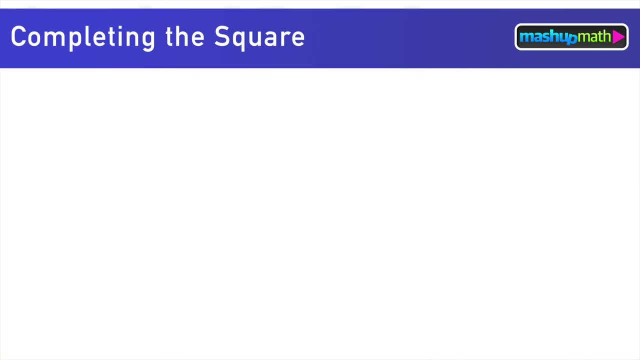 two answers. Now, what's really cool about completing the square is that this method will apply to solving any quadratic equation, So let's go ahead and use it in some more advanced examples. So for our first example, we're going to take the square root of 25, and we're going to 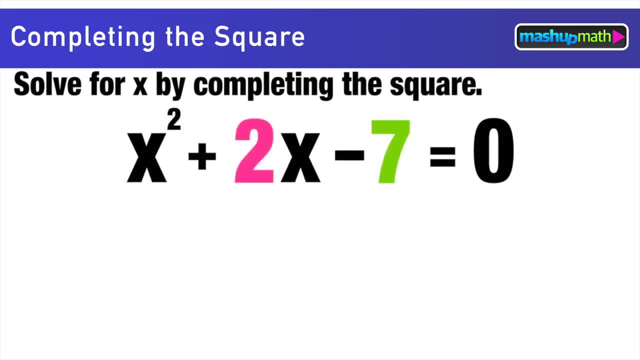 solve for x by completing the square and we have the quadratic. x squared plus 2x minus 7 equals 0.. Now remember, the first step is to rearrange the quadratic so that all the constants are on the right side of the equal sign. So I have to move that negative 7, just. 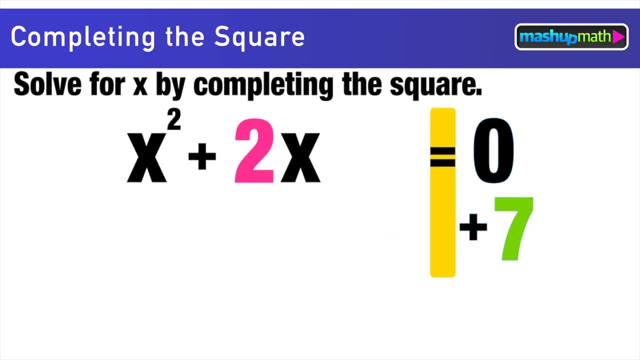 add it to the other side. that'll cancel it out, and now I have x squared plus 2x equals positive 7. Leaving ourselves some room to work with, we move on to the second step for completing the square: taking b over 2 squared and adding it to both sides of the equation. 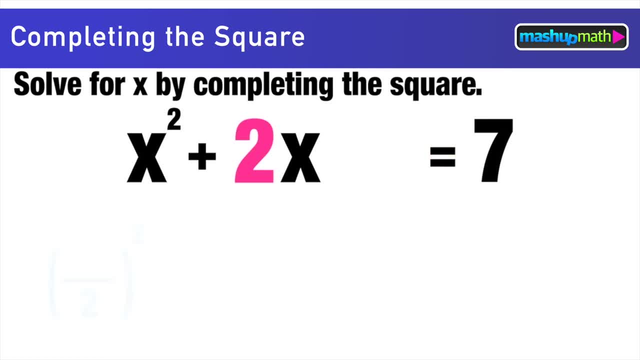 So again I take the b term, divide it by 2, and square it. In this case the b term is 2.. 2 divided by 2 is equal to just positive 1, and we know that positive 1 squared equals. 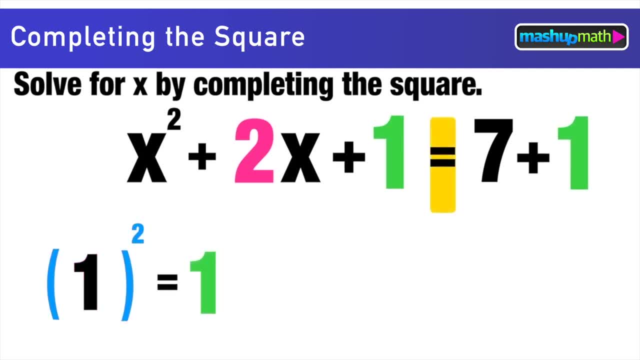 1,. so we're going to be adding 1 to both sides of the equal sign. And now we're ready for the final step: to factor and solve for x. So, just like in the last example, we're going to start on the left side of the equal sign. 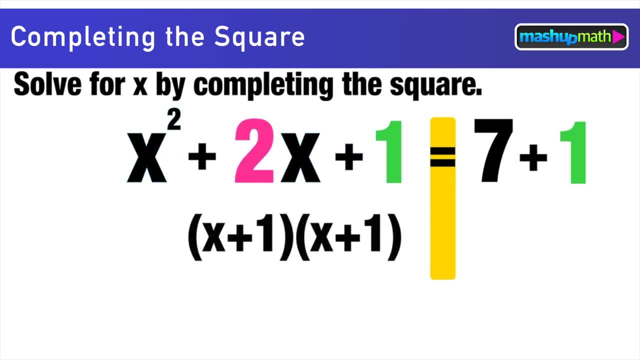 factor that trinomial x squared plus 2x plus 1, which is x plus 1 times x plus 1, when factored out and 7 plus 1 on the right side equals 8.. Now back to the left side: x plus 1 times x plus 1 again. 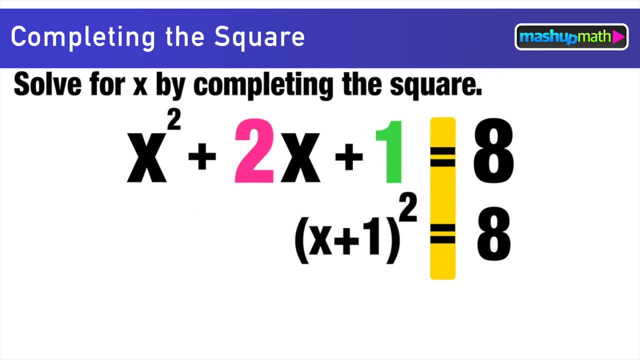 we're going to rewrite this as the sum of x plus 1 squared, and now we can take the square root of both sides. Taking the square root on the left side will cancel out the exponent. the square root symbol and the exponent of the two cancel each other out. Now, 8 is not a perfect square, so I'm 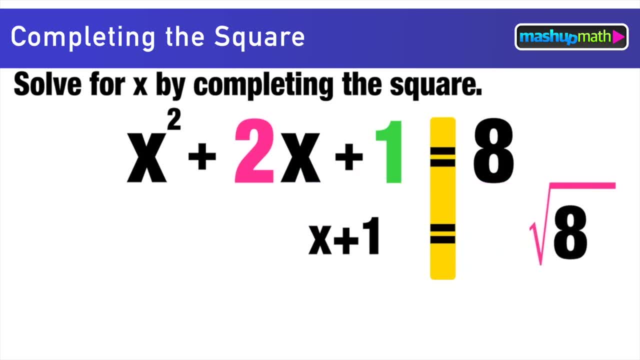 going to leave it in the square root. I'm not going to evaluate it, I'm just going to express it as plus or minus, whatever the square root of 8 is, and then I can go ahead and subtract 1 from both sides. So now I have x all by itself and I'm ready to evaluate to find the two solutions to. 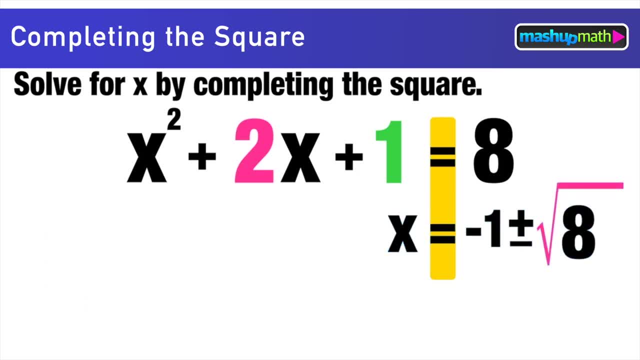 this quadratic. So I have: x equals negative 1 plus or minus the square root of 8.. Now I can evaluate the square root of 8 to approximately 2.83 and then find my two solutions for x Negative 1 plus 2.83 is 1.83.. 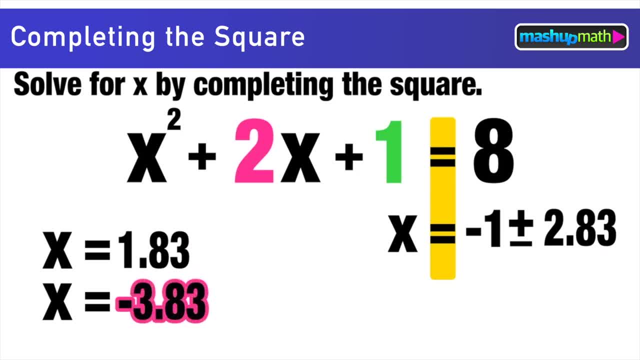 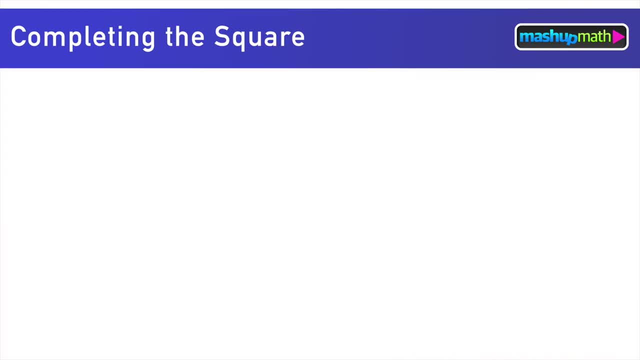 And our second solution: negative 1 minus 2.83 equals negative 3.83, and we have successfully completed the square for this example. Okay, so now we have one more example here where we are going to solve a quadratic for x by completing the square. So in this case we have x squared. 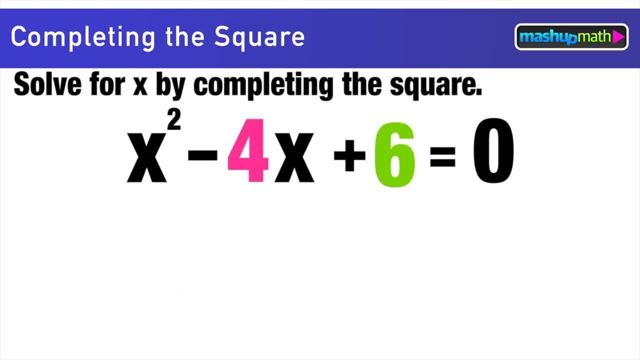 minus 4x plus 6 equals 0.. We have to rearrange it by subtracting that: 6.. Okay, again we want all the constants on the right side of the equal sign. So now we should have: x squared minus 4x is equal to negative 6.. Now we're ready for step 2, which is adding b over 2 squared to both. 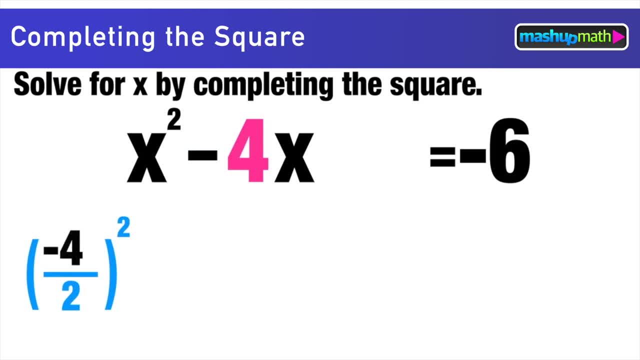 sides of the equal sign. In this case, the b term is negative 4.. Negative 4 divided by 2 is negative 2, and negative 2 squared is positive 4.. So we're going to be adding 4 to both sides of the equal. 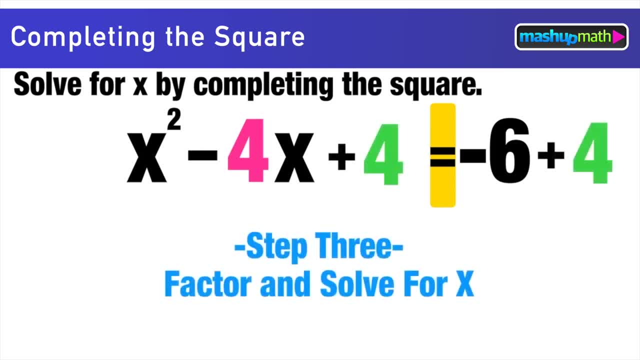 sign. And now we're ready for the final step, which is to factor and solve for x. So start on the left side of the equal sign, the trinomial x squared minus 4x plus 2.83.. And now we're ready for the. 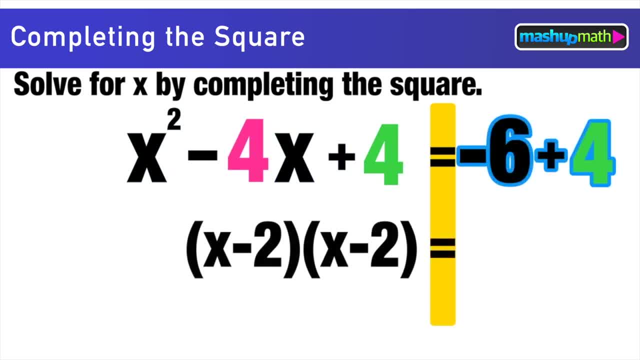 square root of x, squared minus 4x plus 4, factors to x minus 2 times x minus 2.. On the right side, negative 6 plus 4 is equal to negative 2.. Back on the left side, we rewrite x minus 2 times itself.